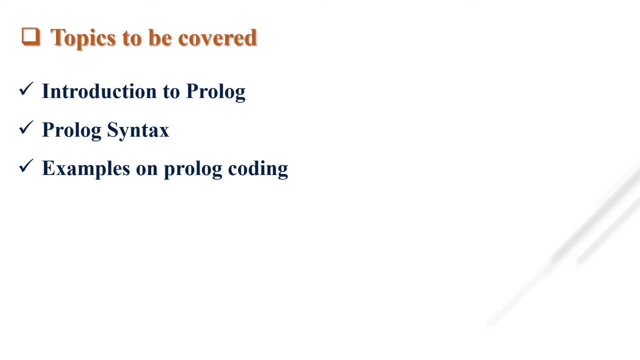 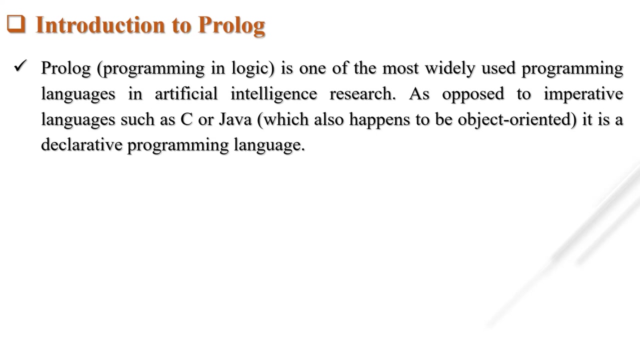 So the topics which are covered in this video are Introduction to Prologue, then the syntax used in Prologue, for example atoms, numbers, values, variables and all, and then we take the examples on Prologue. So Prologue, the full form of Prologue, is Programming in Logic. 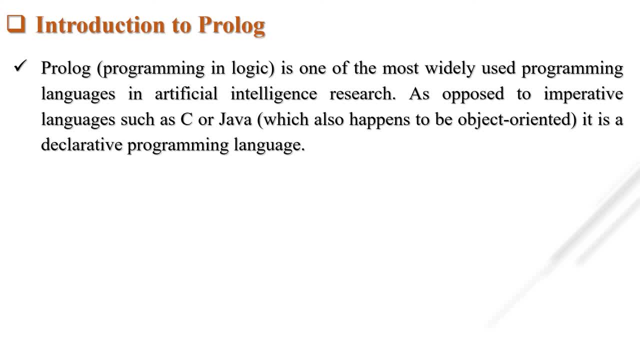 Prologue is one of the most widely used programming language in Artificial Intelligence research. As opposed to imperative language such as C or Java, which also happens to be object-oriented, it is declarative programming language. That means when implementing the solution to a problem instead of specifying how to achieve a certain goal in a certain situation. 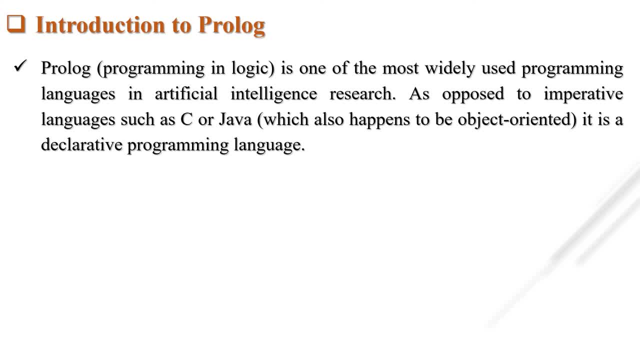 we specify what the situations and the goal are and let the prologue interpreter derive the solution for us. So prologue is very useful in some problem areas like Artificial Intelligence, natural language processing, database, but pretty useless in others like graphics or numerical algorithms. 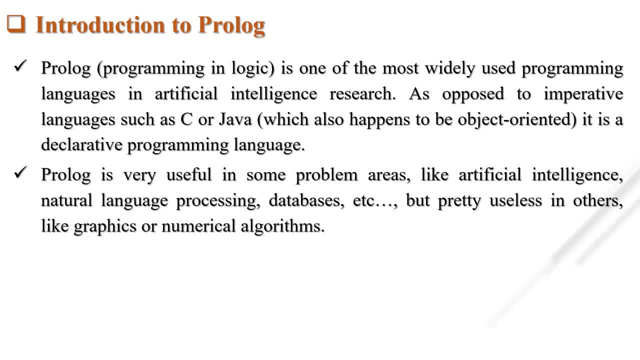 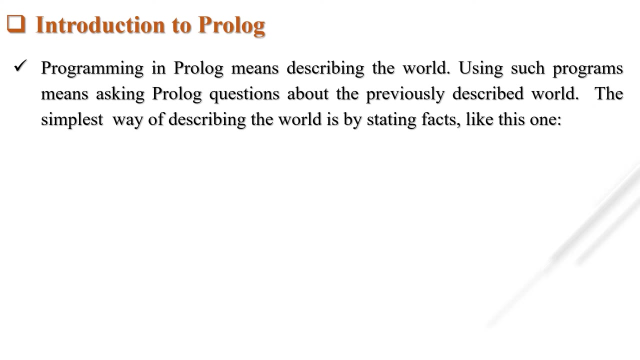 By following this unit, firstly, you will learn how to use Prologue as a programming language to solve certain problems in computer science and Artificial Intelligence, And secondly, you will learn the prolog interpreter actually works. so let's proceed with the prolog. so programming in prolog means describing the world. 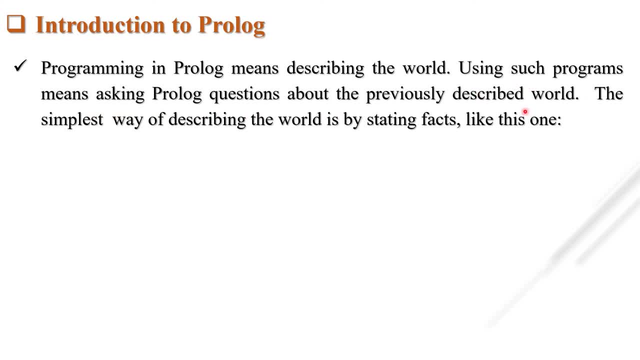 using such prolog means asking prolog question about the previously described world. so the simplest way of describing the world is to stating the fact. like this, one like bigger in the opening bracket, elephant, comma horse. so this paid the fact that an elephant is bigger than a horse. whether the world disturbed by a prolog program has. 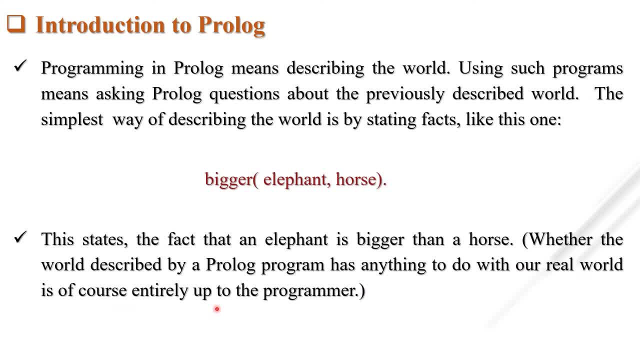 anything to do with our real world is, of course, entirely up to the programmer. okay, so we previously described all the things in our coding and then we asked the prolog: that Is elephant? Yes, elephant is. 자�ji is bigger than horse. then they simply gives the answer like yes or no. okay, 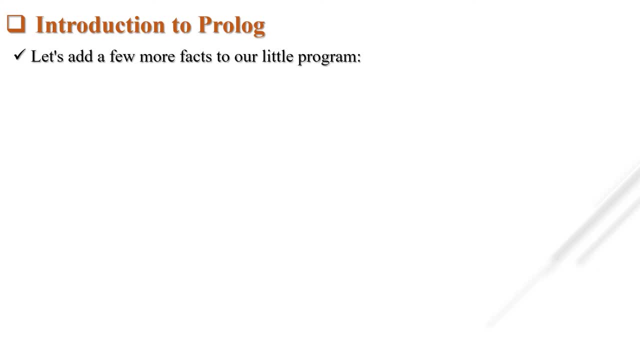 so let add a few more facts to our later program. like the fact is, elephant is bigger than horse. next, horse is bigger than donkey, donkey is bigger than dog, donkey is bigger than monkey. so this is all upon the programmer whether he described the fact. 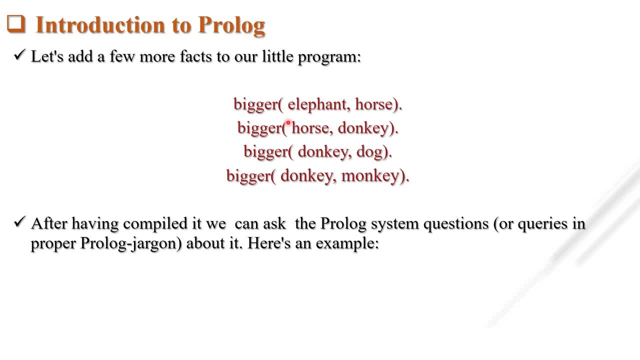 is true or not, otherwise the prologue is going to be give the answer as a false. so after having compiled, if we, if we ask the prologue system questions or queries in the proper prologue jargon about it, here's an example. suppose i ask: is donkey is bigger? 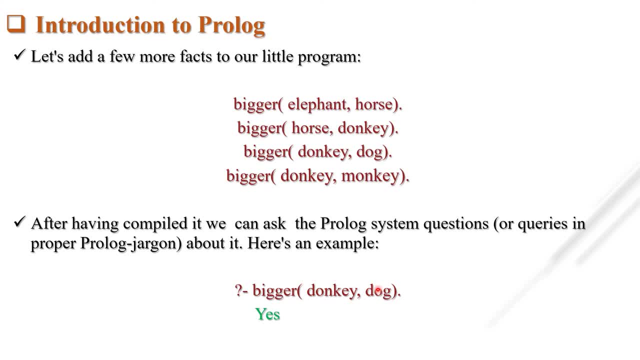 than dog. so they reply us that yes, donkey is bigger than dog. why? because we already described this. okay, suppose you uh. suppose, when we uh, when you ask a google assistant that who is the prime current prime minister of india, the system gives the answer that narendra modi is the current prime minister of india. 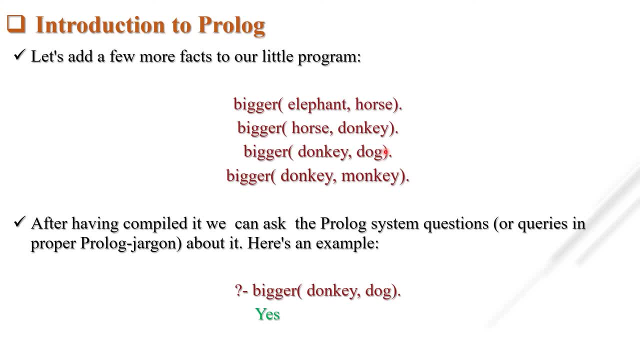 but if you ask that who is the prime minister of india in 2025 or 2030, then the system are not able to give the proper answer. why? because they does not have any database of fact. okay, so when you ask to google assistant that like, what is the current temperature? 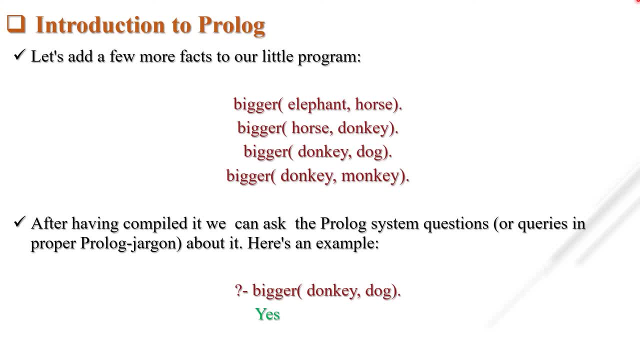 in a particular state or particular city, they will give you because they already have the data. okay. so this is completely depend upon the programmer. if they- uh, if they state true things in the database, then, and only then, you can get the perfect or true things as a output. 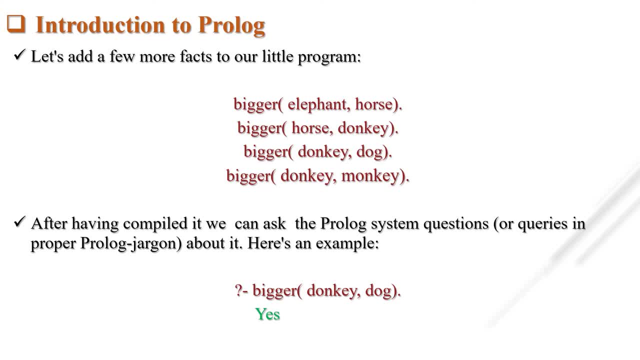 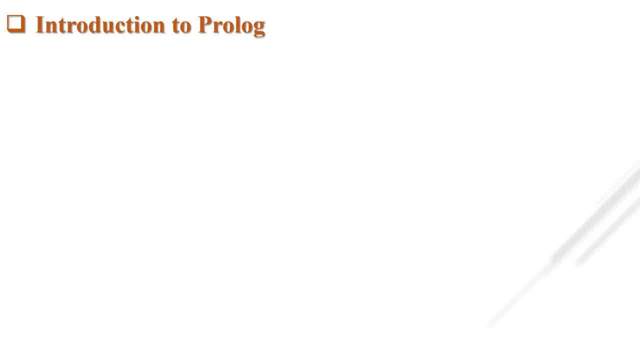 okay, if i write dog is bigger than donkey, then it is false. it is a mistake of programmer, not the google assistant or not the artificial intelligence. okay, suppose the query bigger donkey dog. okay, donkey is bigger than dog. that is the question is: a donkey is bigger than dog succeeds. 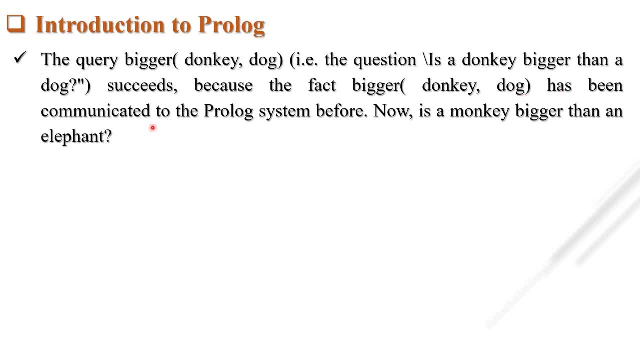 because the fact bigger donkey comma dog has been communicated to the prologue system before now- is a monkey is bigger than an elephant. the system give the answer no, because this is not in our database, not in the fact. also it is not a fact and also it is not in our database. okay, so the question is that how? 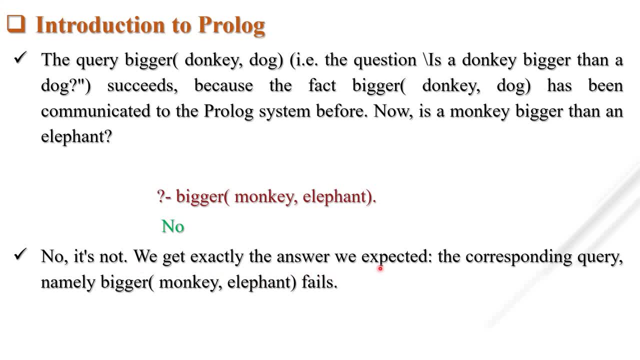 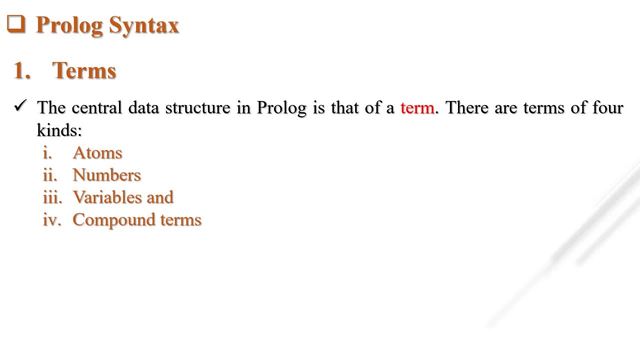 we get the answer. so not, it's not. we get exactly the answer we expected. the corresponding query, namely bigger monkey elephant, fails because we are not mentioning that in our database. so let's proceed with the second public, that is, prologue syntax. that is most important before proceeding the prologue coding. so the central data structure in prologue is that of term. 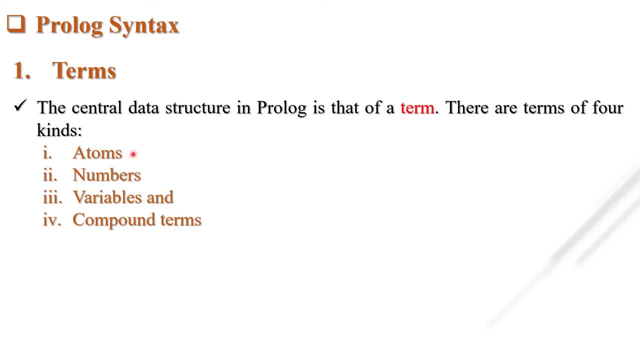 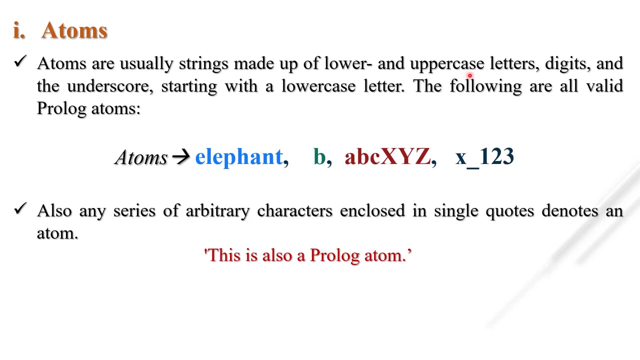 there are. there are terms of four kinds: first one is atoms, second one is numbers, third one is variables and fourth one is compound. so what is atom? atom are usually string made up of lower and uppercase Letters, digits and the underscores. starting with the lowercase letter, the following of the valid prologue: 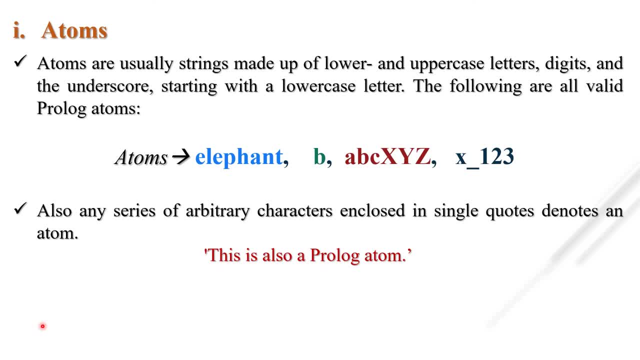 atom. okay, so how we declare or initialize with the atoms. it must be a list, sang� sgitmanpl, lowest letter first, and it is the combination of 1, 2, 3 up to 9, 0 to 9. also we can use upper case. 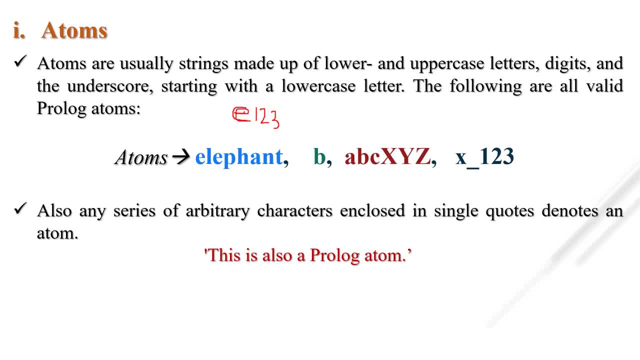 but the first letter must be lower in lower case. okay, so this is a valid atom. this b is also valid atom. a, b, c, x, y, z is also valid atom. x. underscore 1, 2, 3 is also valid atom. so the atom always proceed with the lower case letter. that you have to keep in your mind. also, any series of arbitrary. 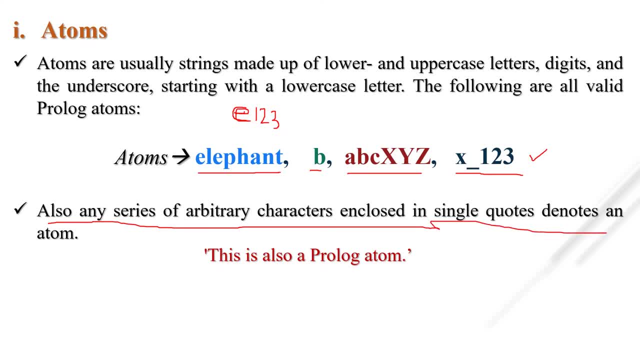 character enclosed in a single quote denotes an atom. okay, so if i write in the single quote 1, 2, 3, then also it denotes an atom because it is enclosed in single quotation. okay, so if i want to make a long string as an atom, then i have to enclosed in a single quotation mark. 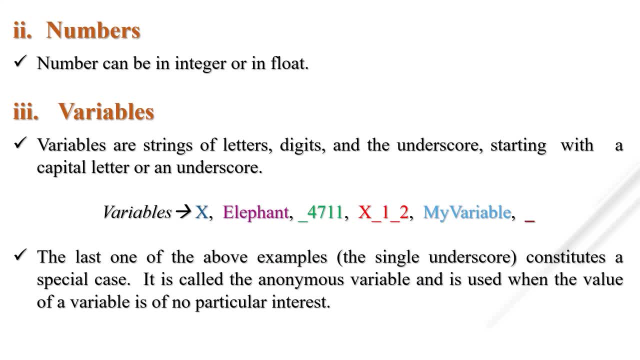 okay, okay, next number: number can be in integer or in float. third, one is variable. now this is also important when you are doing a prologue coding how we can declare the variable. so variables are the string of letters. letters includes upper case letter and lower case letter, digits and the underscore, but it start with a capital. 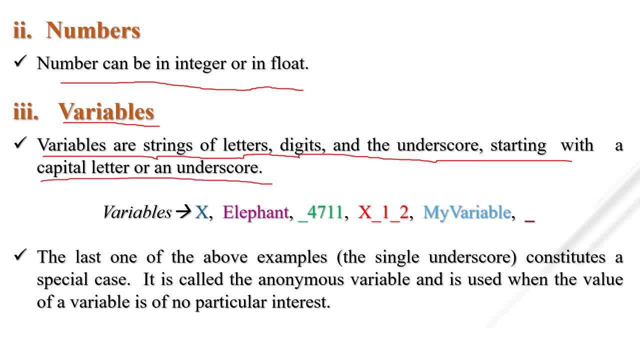 letter or an underscore, just like a, c in c. we can start with the and we can start our variable name as uh, with the underscore or capital letter, capital letter or small letter. but here we can mandatory, we have to start with the capital letter. so these are the valid variable name. for example, first one is x. this is also valid. 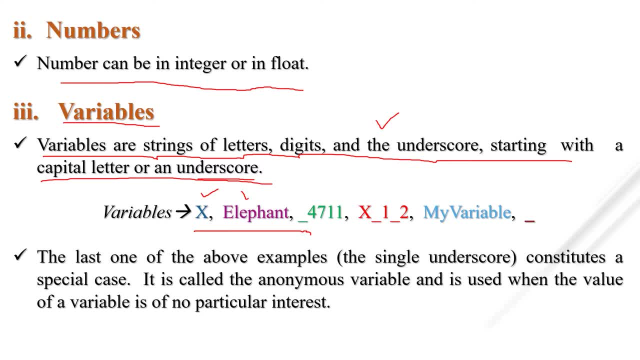 because it start with the capital letter. then this elephant- this is also start with the capital letter, and this underscore 4711 is also valid. okay, our variable is a valid في variable because it starts with the underscore x. underscore 1 score is also valid. my variable is also valid and this underscore 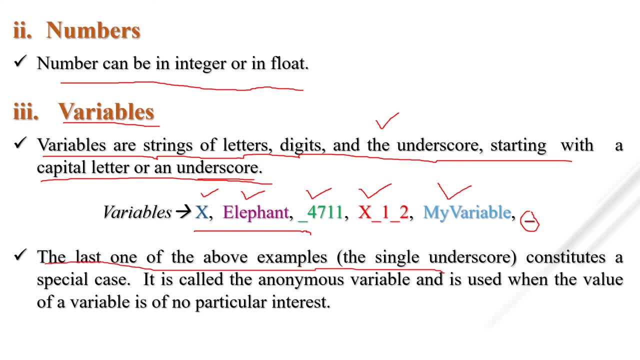 only underscore is also valid because it has some meaning. the last one of the above example, that is, the single underscore, constitute a special case And is used when the value of variable is of no particular interest. Suppose I have used this variable, but I am not using this variable as a printing any number or any character. 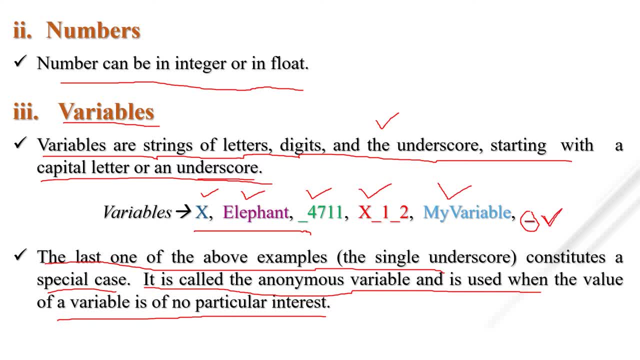 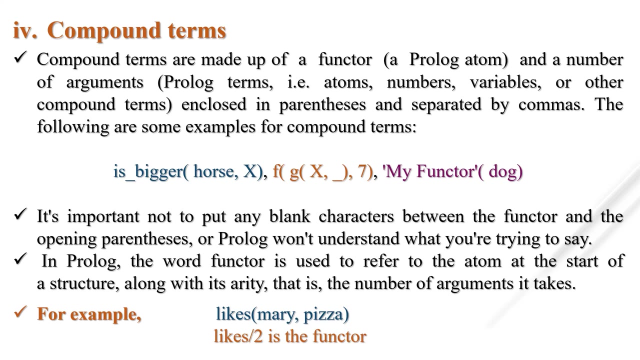 Then, and only then, I can use only underscore. Okay, This is an anonymous variable, So we can rewrite the numbers or characters on it, But we are not going to use that particular variable. Then we can use this underscore, Okay. The fourth one is compound term. 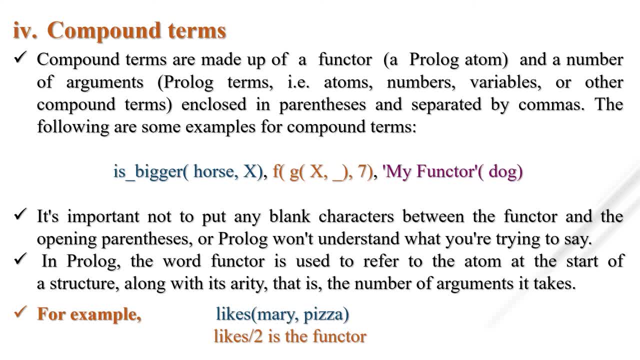 So compound terms are made up of functor- It is also known as a prologue atom- And a number of arguments. It includes prologue terms, that is, atoms, numbers, variables or other compound terms, Which is enclosed in the parenthesis and separated by commas. 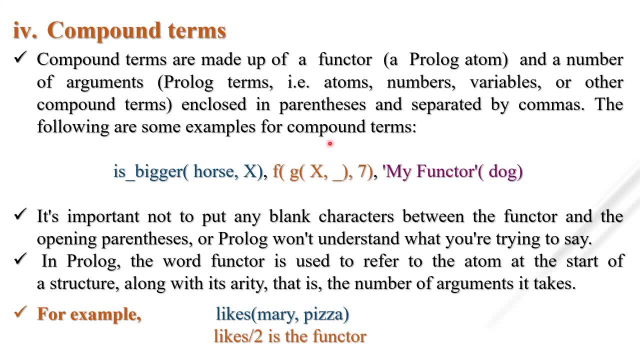 So the following are some examples for compound terms. For example: is bigger in the bracket horse comma x. What this means horse is bigger than x. What is x? X is a variable. Horse is an atom. Okay, I already told you that argument we can use as a prologue term. 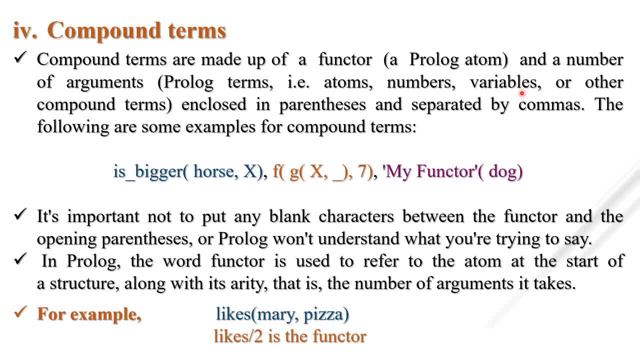 It may include atoms, numbers or variables. Okay, Comma f of g x comma, anonymous variable, that is underscore comma seven, My functor. This is also an atom, I already told you. It may be start with capital letter, But it is enclosed in single quotation mark. 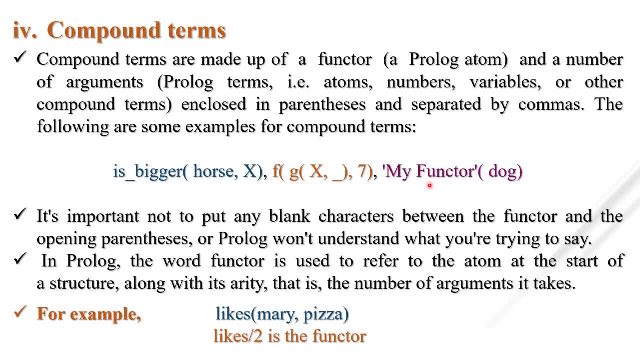 That's why this is denoted as an atom. This is an argument which denotes an atom. So combination of all three- All three means atoms, numbers and variables- is a compound term. So it is important not to put any blank character between the functor and the opening parenthesis. 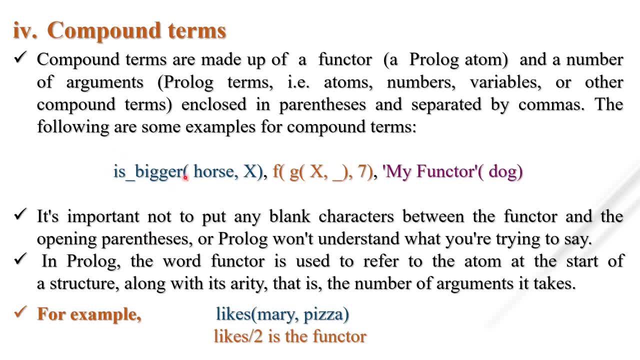 So this is also known as functor. This name before this opening bracket is known as functor. For this, g is a functor. For this, all f is a functor. Okay, Our prologue won't understand what you are trying to say, So we have to take care that after this functor, 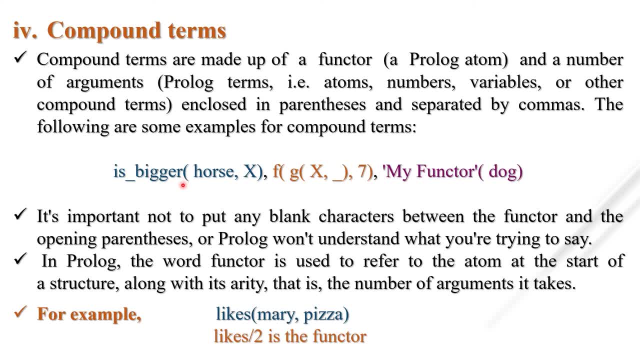 we don't have to specify any blank space. so in prologue the word functor is used to refer to the atom at the start of a structure, along with its arity. that is the number of argument it takes. for example, if i like, like, if i write likes in the 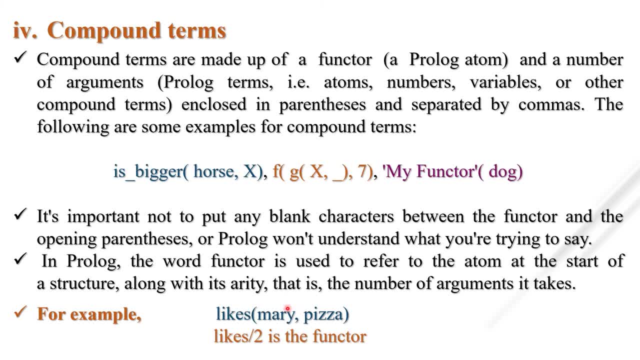 bracket: mary comma pizza, then how we can see this? mary likes pizza. okay, so likes is a functor which have two argument. okay, this like is a functor which have two arguments, so this is known as functor. functor have one parameter, that is number of argument which are used in likes functor. okay, 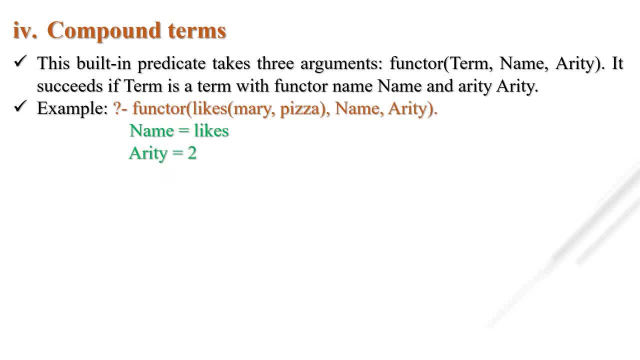 let's see an another example. so the built-in predicate takes three argument. this is a built-in uh predicate that we can use you at the prologue console. so if we write functor term, name and arity, it succeed. if term is a term with functor name, capital name and arity arity. for example, if i write functor likes in the bracket. 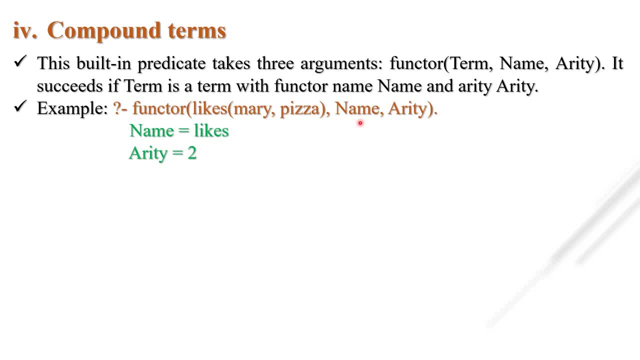 mary comma. pizza comma. name and arity. so name is a variable, so name includes like, the name of functor is likes and uh, how many parameter we can uh, here we are using this two. that's why arity is a変 to and we were talking about. so they are called classłem. 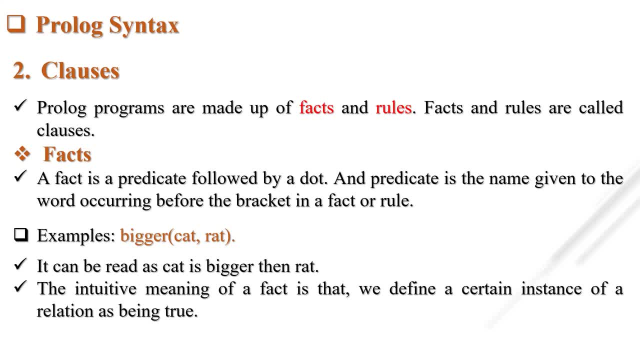 is month and pas dare is another one. so basically say one where they are y cross, so this becomes pros removed. so the answer is: plus fire says cause, plus capital state is equal to one. now if i ignore plus, you would over come right. and i know, yes, and i know also this is: 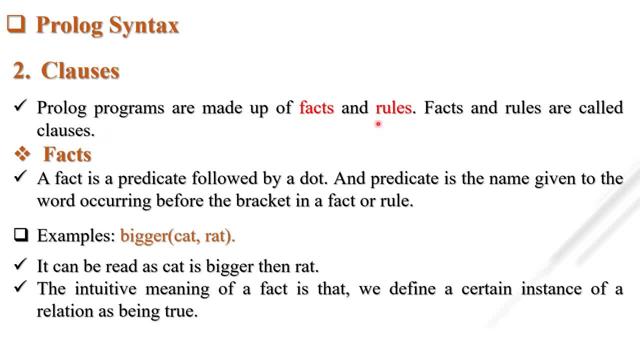 marry someone else? if i over talk, the answer is not correct. yeah, so this is possible, even if we are acting on like in the bracket and let's say, add fn. so if i try vario then it would be Lithium and� what is fact and what is rule? okay, so fact is a predicate followed by a dot. 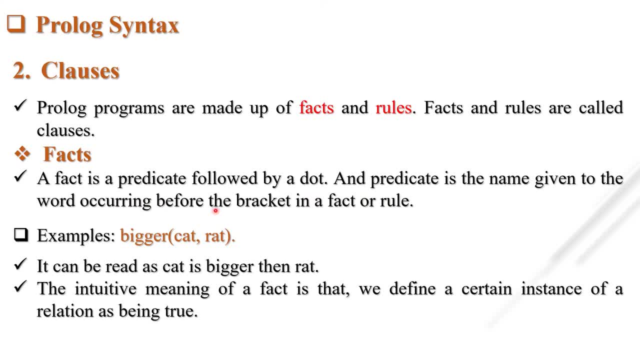 and predicate is the name given to the word occurring before the bracket in a fact or rule. for example, bigger in the bracket: cat, comma red. at last we have to put a dot. so this is a fact, that cat is a bigger than red. okay, so the intuitive meaning of a fact is that we define a certain instance of a relations. 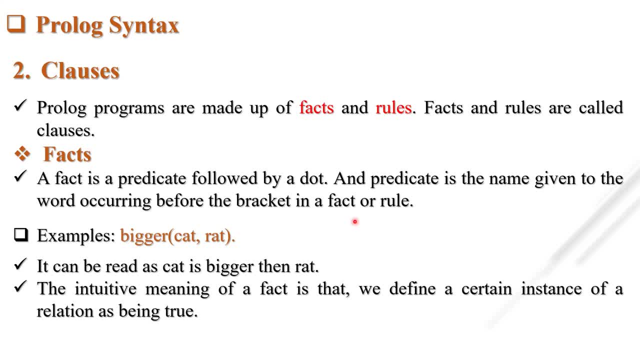 as being true. for example, i can write first prime minister of india. in the bracket i can write jawaharlal. okay, so that is a fact that we can mention in our database. but they have some rules that a fact is a predicate followed by dot. we have to put a dot and it is a variable. 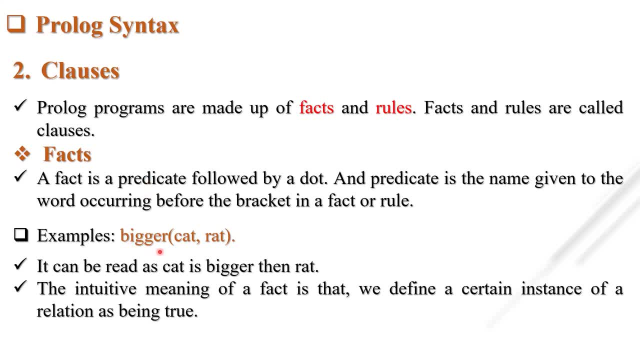 put a dot. and what is this predicate? this functor is also known as predicate and the predicate is the name given to the word occurring before the bracket. that's why this is known as functor. also, this is known as predicate before the opening bracket. whichever we- uh, we are giving the name as an atom is our predicate. 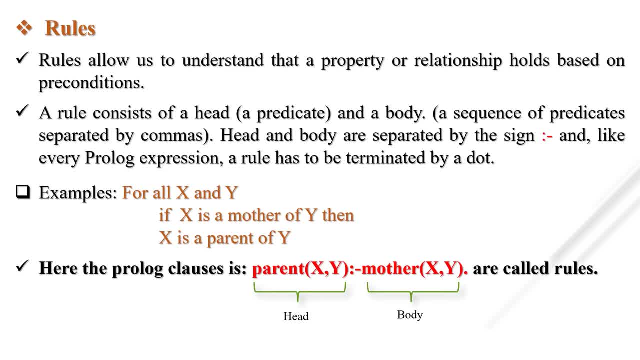 pre ans. then what is rule? fact, we know that a predicate which followed by a dot. it is known as fact. but what is rule? rule allow us to understand that a property of relationship holds based on the preconditions. so a rule consists of a head- that is, a predicate- and the body. 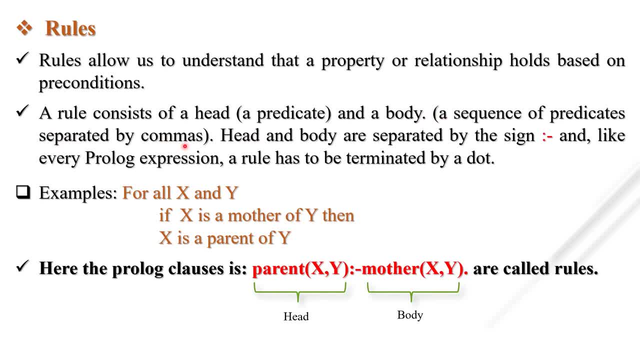 body. what is body? accomplices, or necessarily among the live objects. so what is body? espíritu? meaningist sequence of predicate separated by comma. okay, so rule is consisting of head and a body. here you can see, this is head and this is body. okay, head and body are separated by sign, this colon, and. 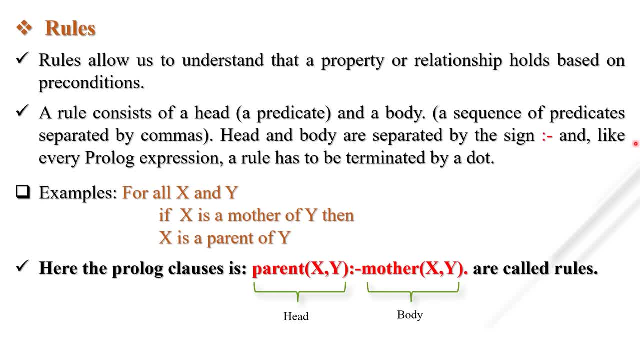 hyphen. okay, we are already putting here. and like every prologue expression, a rule has to be terminated by a dot, so we have to put dot here. suppose we are taking one example, that for all x and y, if x is a mother of y, then obviously x is a parent of y. so, when we can, when we can say: 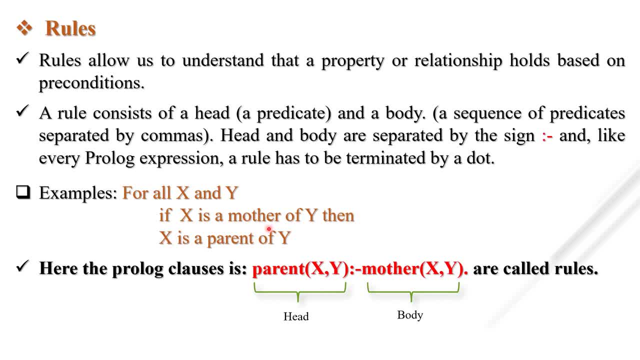 that x is the parents of y. if x is a mother of y or x is a father of y, or x is a brother of y or x is a sister of y, then, and only then, we can say that x is a parent of y. okay, so how we can write in the prologue that parent x is a parent of y if, and only if, x is a. 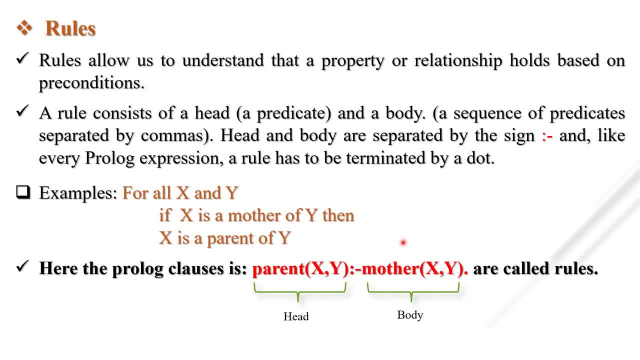 mother of y. so if this body is true, then, and only then, this head is going to be true. so it have some preconditions, but in fact there is no precondition. we have to check, we have to only mention this: this is a bigger than this, or this is a prime minister of. 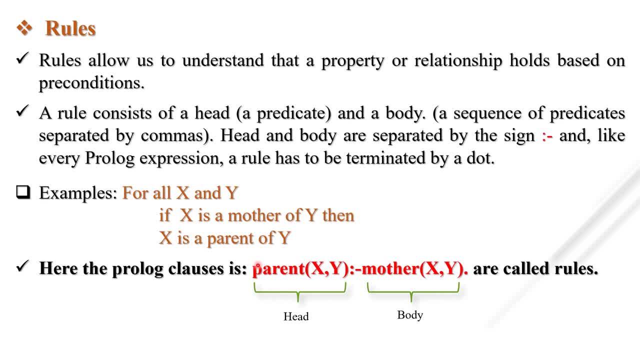 uh first feminist of india. is this also we can say that? uh, abhishek bachchan is a child of abhis amitabh bachchan. that is a fact. okay, so in rules there is a precondition to fulfill this head. when we can uh, when the prologue gives yes, when uh x is a mother of five, then, and only then, the 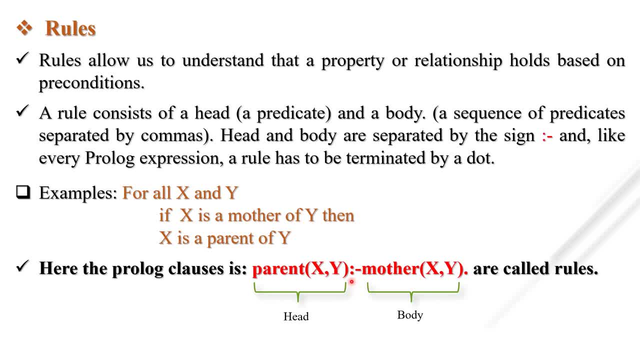 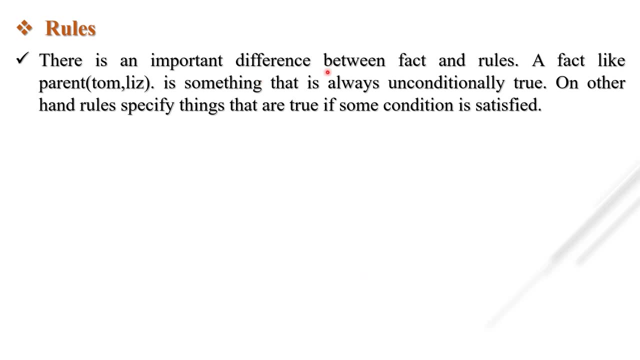 prologue says yes, the for x is a parent of y, so this is known as rules, which consist of head and body, and it will be separated by colon and hyphen. so there is an important difference between fact and rules. fact, like parent tom comma lease, is something that is always unconditionally true. 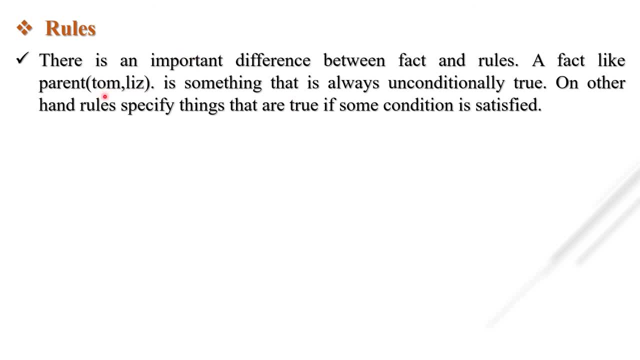 there is no condition before this, so i can say that amitabh bachchan is a parent of abhishek bachchan. it is true, so it is a fact, unconditionally true. there is no condition, uh, to prove this. on other hand, rules specify things that are true, if some. 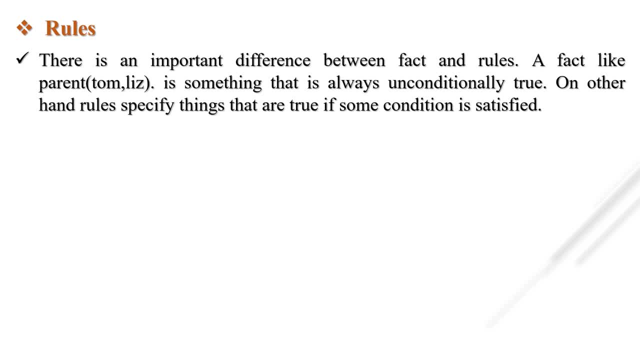 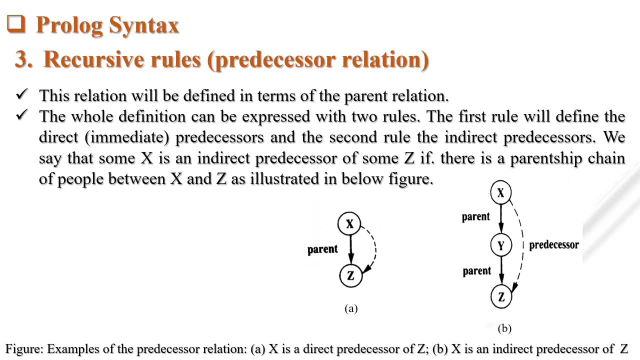 condition is satisfied. okay, if body is satisfied, then only it will be satisfied, otherwise not so. next one is recursive rule. that is also known as predecessor relation. so this relation will be defined in terms of parent relation. the whole definition can be expressed with two rules. first one is the first rule will be defined: the direct, that is, immediate predecessor, and 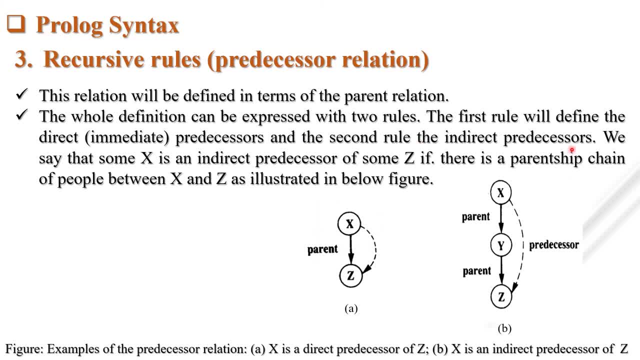 the second rule: indirect predecessor. this is known as direct predecessor, this is known as indirect predecessor. okay, we say some x is an indirect predecessor of z. if there is a parentship chain of people between x and z, okay, here is a parentship chain that x is. 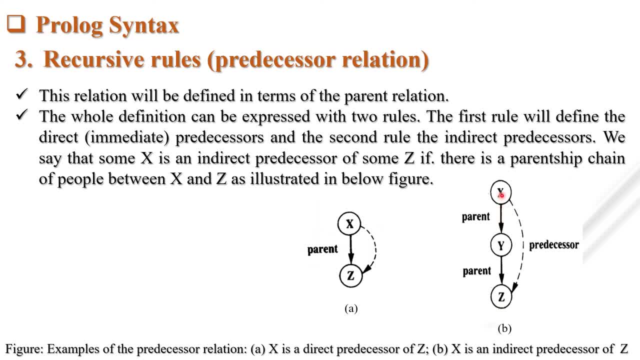 a parent of y and y is a parent of z, then we can say x is a predecessor of z. also x is a parent of z. okay, but this is a first rule that defines immediate, that is direct predecessor. x is a directly- uh, direct predecessor of z. here x is an indirect predecessor of z. 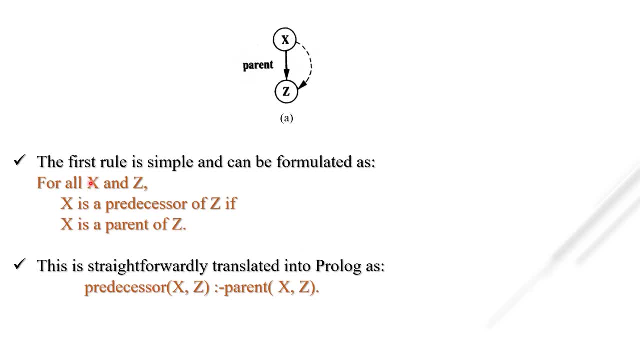 okay. so the first rule is simple and can be formulated as for all x and y: x is the predecessor of z if x is a parent of z. so, with the help of rule, what we can, uh, what we write as a prologue syntax: x is a predecessor of z if x is a parent of z. okay, this is going to be true when, when this is. 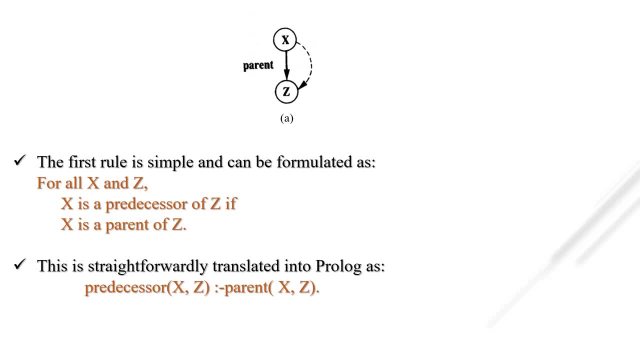 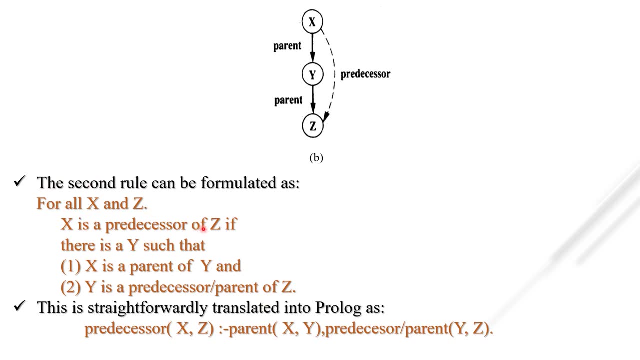 going to do. the second rule can be formulated as for all x and z: x is the predecessor of z if there is a y, such that x is a parent of z and y is a predecessor or parent of z. so how we can translate it as a prologue: x is a predecessor of z if x is a parent of y. 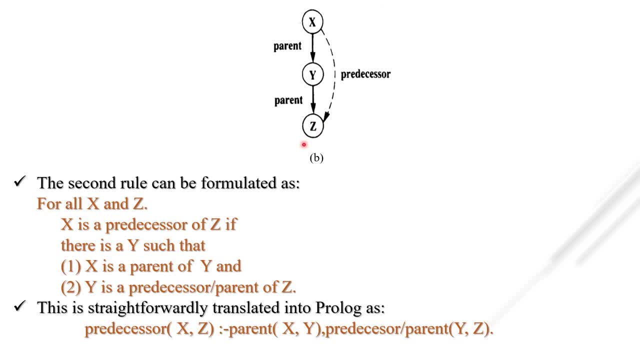 and y is a parent or predecessor of z, then, and only then, we can say: x is a predecessor of z. so we, if this two rule going to be succeed, then, and only then, this head, that is x is the predecessor of z, is going to be succeed. otherwise, 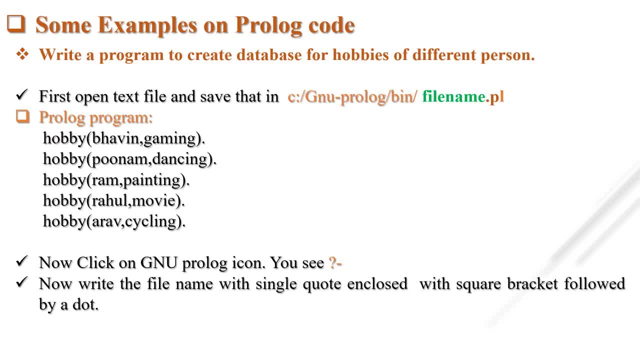 not. so now we are going to see some examples based on prolog coding, so this is also helpful in the laboratory. so how to create a prologue file? that first we are. first i am going to explain that. first you have to open one text file and save it in c colon- gnu prologue. in gnu prologue, you have to open the folder bin. 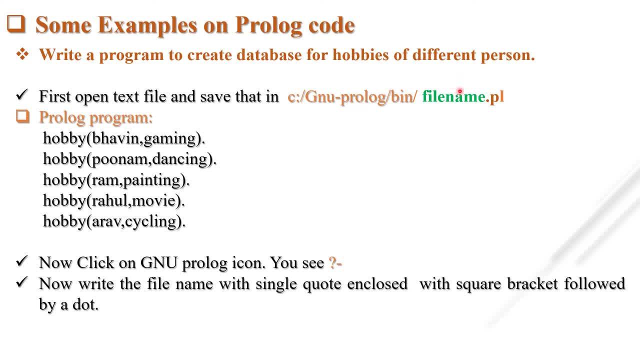 and then you have to give a particular this file, particular file name with extension pl. that is programming logic. so first you have to install gnu prologue, then, and only then, you can locate this folder. okay, suppose i open and my file name is one dot pl and i write the prologue. 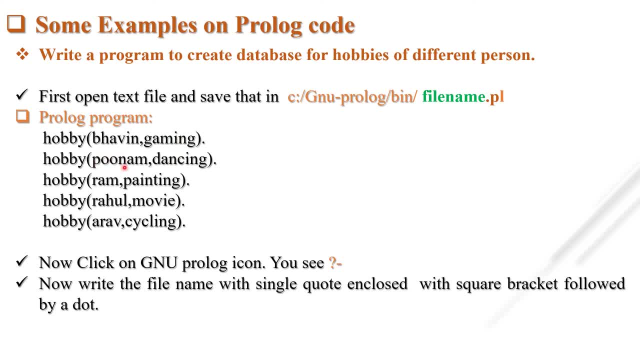 program that bhavin's hobby is gaming, punam's hobby is dancing, ram hobby is painting, rahul hobby is movie watching movie or aro hobby is cycling. okay, then i close that particular dot pl file. then i have to click gnu prologue icon. 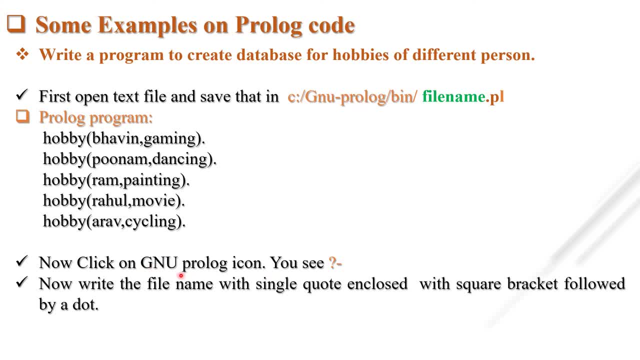 okay when, when you install gnu prologue, uh, on the desktop you have an icon of gnu prologue. whenever you double click or single click on gnu prologue, you can see that question mark. now you have to write a file name to compile. for compilation, you have to write a file name that is 1.pl, with a single code, and it must be. 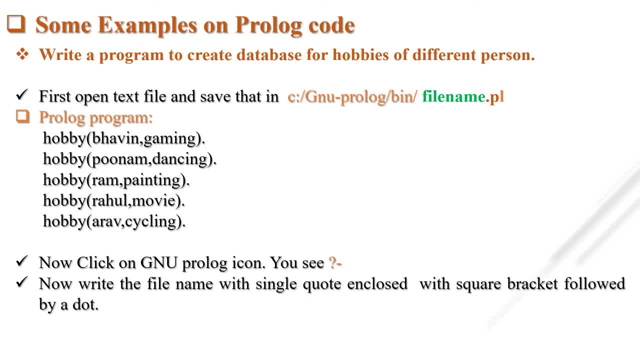 enclosed with a square bracket followed by a dot. for example, i have a file name 1.pl. then after question mark i have to write in the single quote one dot, pl. single quote. over closing bracket it must be followed by a dot. then a program is going to compile with the help. 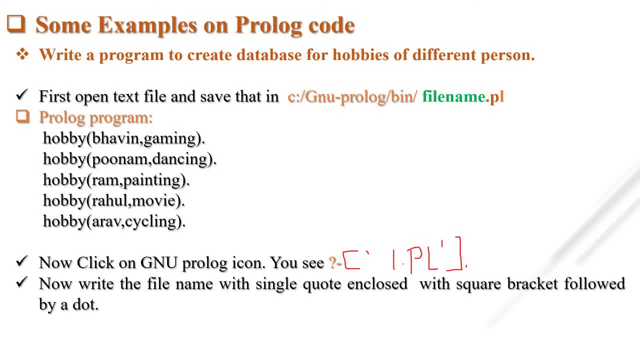 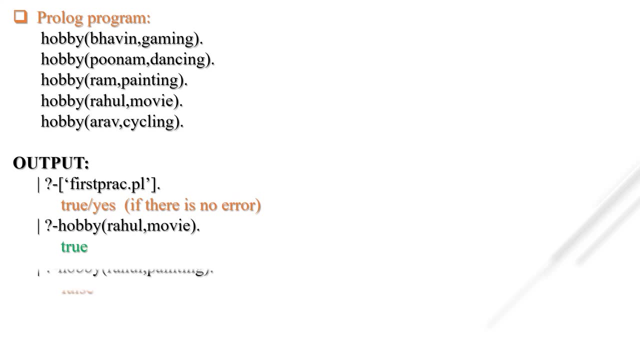 of prolog, gnu prolog. if there is any error, it will display you. otherwise you can ask the program on the basis of this coding. suppose our compilation succeed, then what so when, when i ask the prolog of query that rahul's hobby is movie, then it will be say: 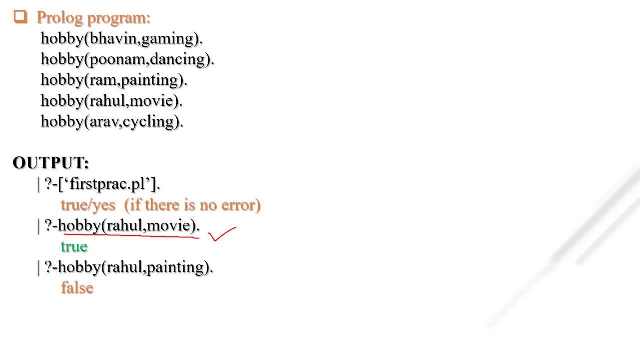 yes or true? and if i ask rahul hobby is painting, then it will say no. how this will be interpreted from top to down. first argument is rahul, no. second argument is rahul, no. third argument is rahul, no. this fourth predicate: 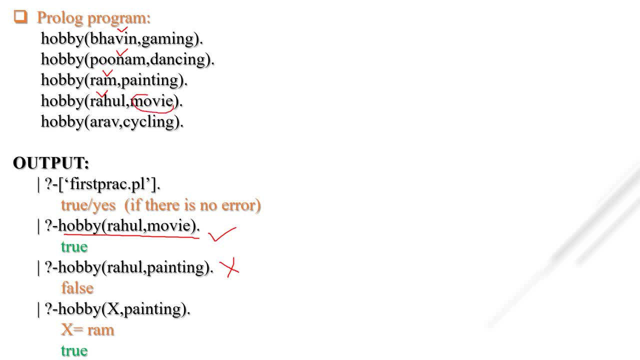 argument says how layers and it will be checked with the second argument. second argument is movie, but here we are writing painting. that's why it says no. ok, if i ask hobby x, comma painting, then once again it will be come from top here: x equal to bhavien, argument 1. argument 2 is gaming. it will not match with the painting, that's. 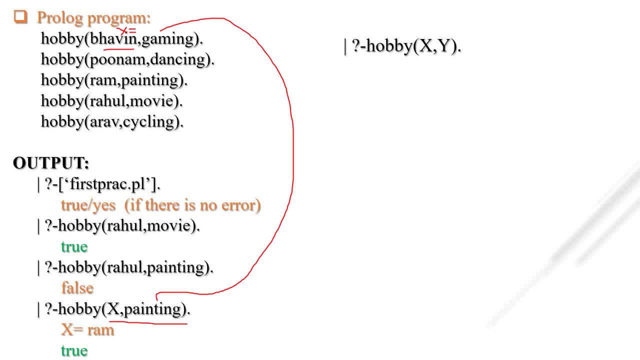 why x. x is not equal to bhave. then second: x equal to poona. but second argument is not matched with this painting. that's why x does not equal to punam. similarly, x equal to ram. and second argument: if second argument is matched, then it will be show you that x equal to ram. 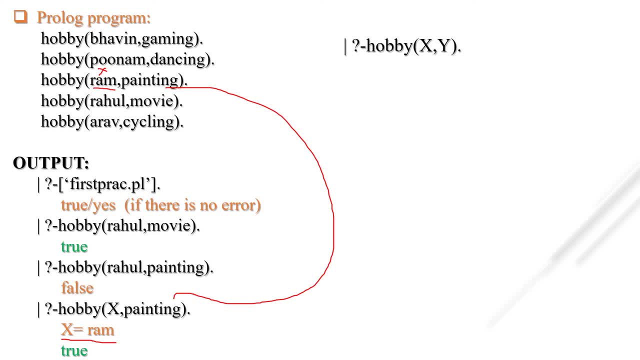 similarly, if i ask hobby x, comma y, both are variable so it will be go from top to down. first word, x equal to bhavin, y equal to gimi, then there is a question mark why it will return question mark because it says you the prologue says you that you have another alternative for. 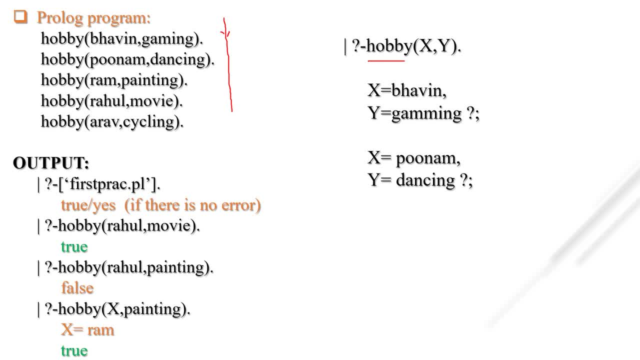 the predicate hobby. what is the next alternative? for to see the next alternative you have to hit semicolon. so if i hit semicolon, then it will give the answer that x equal to punam and y equal to dancing. similarly, once again there is a question mark because there is another alternative for hobby. 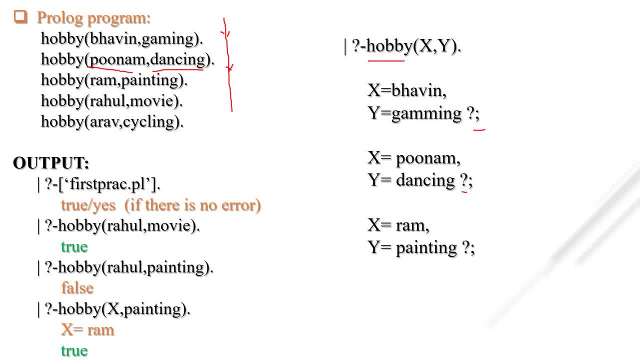 from if we go from top to down. so if i hit semicolon, then x equal to ram and y equal to painting. similarly, x equal to rahul and y equal to movie, and it will be stopped when x equal to and y equal to cycling. okay, i hope you understand this. huh, this is most important. 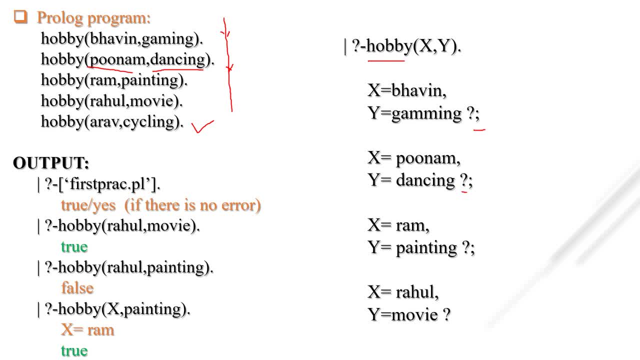 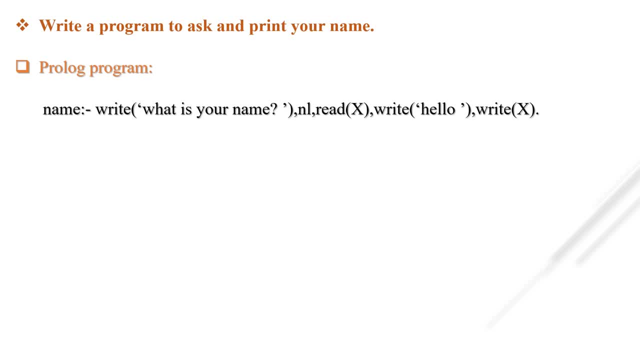 how argument values are replaced you can see here. so next program is to ask and print the name with the help of prologue. so always you have to start whenever you want to ask the or enter the particular character or particular string from the keyboard. then you have to start with any one of the atom. 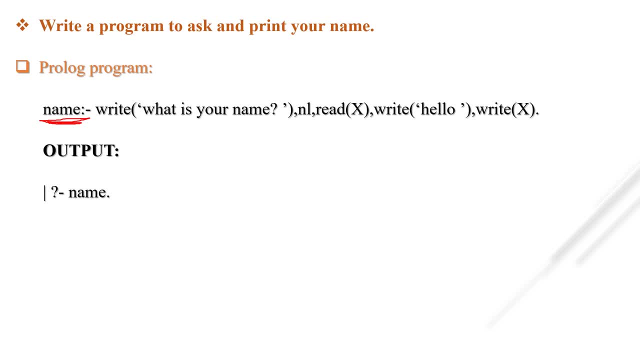 suppose i am using an atom name, then i have to write colon and hyphen. then, similarly, similar to java for printing, we are using write. okay, write in the single quote what is your name. this nl indicates new line and read indicates it scans the string from your keyboard. just. 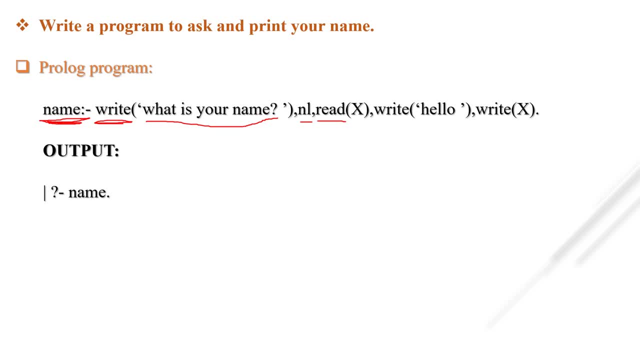 like a scanf in c. so i read from the keyboard that are stored in variable x. then i write hello, hello, hello, hello, hello, and whatever we stored in x will be printed. next let's see the output is: if i hit name dot, this is a particular atom dot. 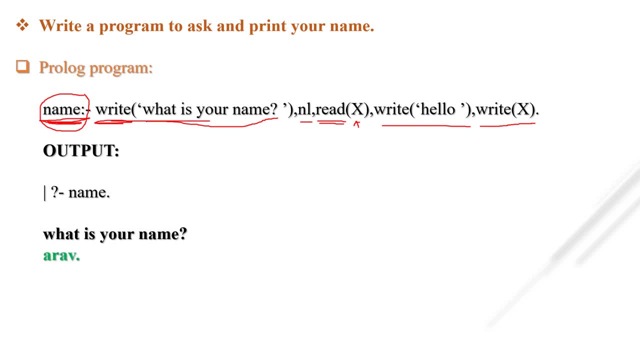 then we what is going to display? what is your name? then read x. suppose i write rou. then full stop. i have to mandatory i over ending the statement. i have to add full stock. if i had full stock Then it will be go to the next line. that is hello and then arrow. Because we have write here, write x. The value of x is arrow. The user inputted the string arrow in variable x. That's why when we write this x, it will be printed as arrow.